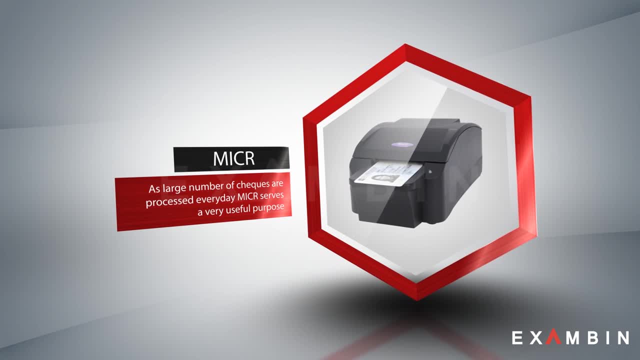 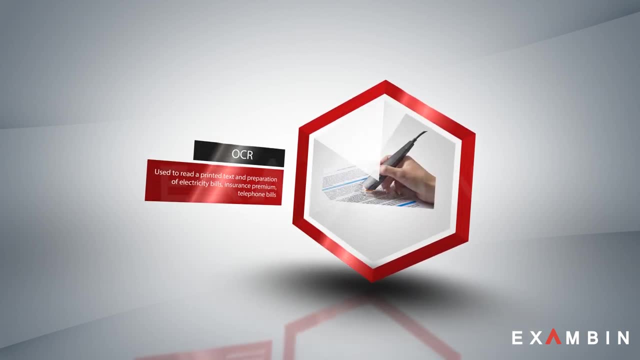 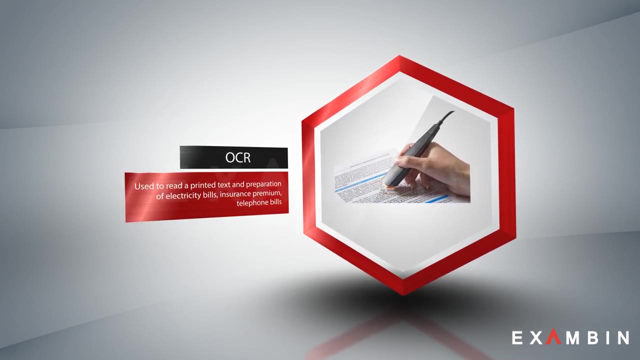 OCR is mainly used to scan and deduct the text inside a image document. Optical character reader: OCR Used to read printed text and preparation of electricity bills, insurance premium and telephone bills. OCR is mainly used to scan and detect the text inside a image document- OMR. 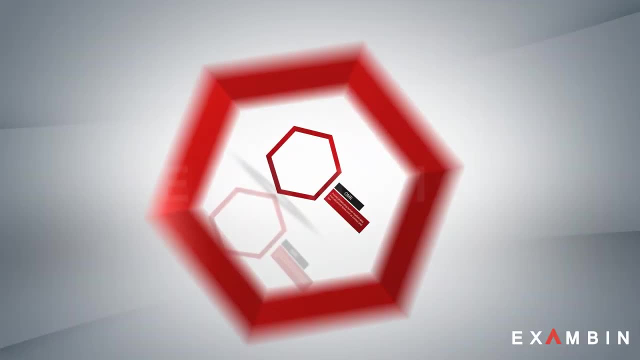 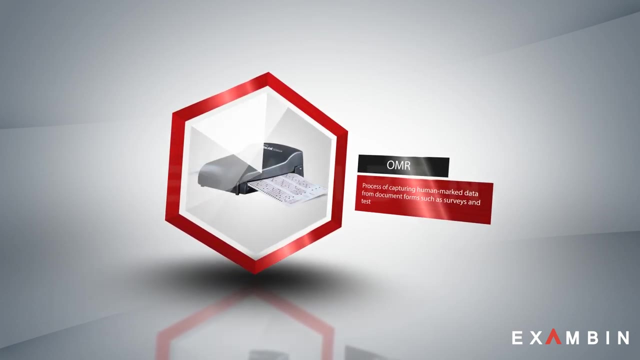 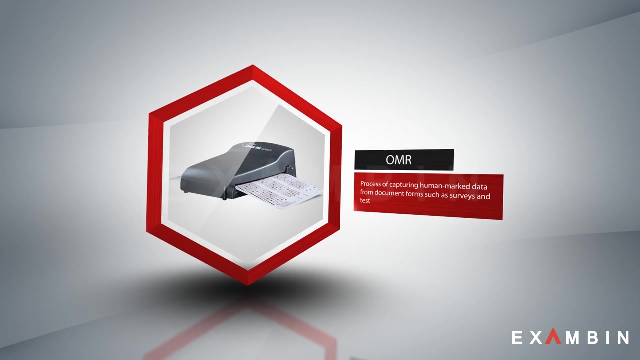 Hi Optical Mark Recognition Process of capturing human mark data from document forms such as surveys and tests. OMR is mainly used in examinations. You can see that OMR sheet where we will be marking options A, B, C, D and all that is. 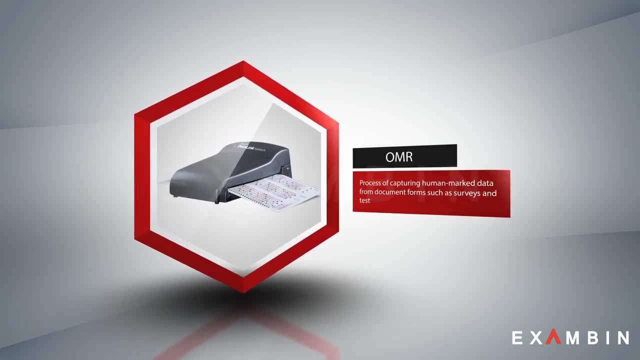 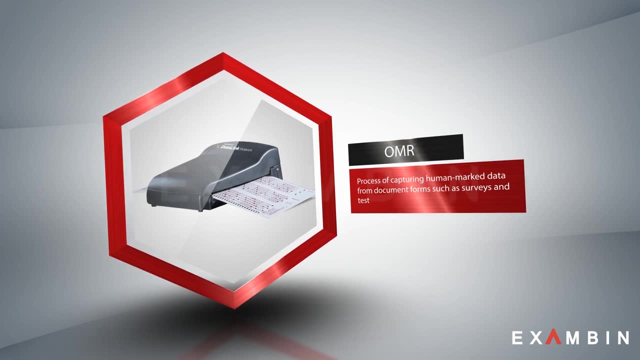 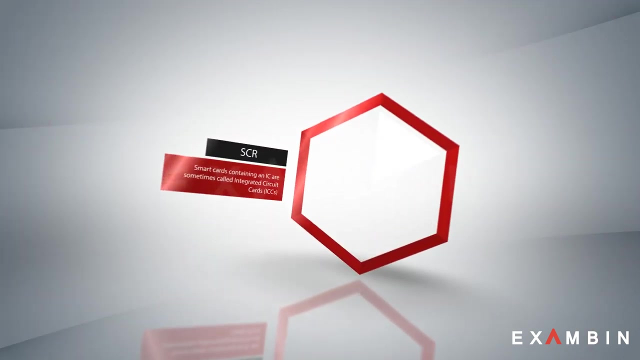 nowadays coming out of patient because everyone going for computer test. But, however, there are still existence of those surveys and polls where agents will be going shop by shop or home to home to take surveys. so those are all processed by OMR only Smart Card Readers. Smart cards containing an IC are sometimes 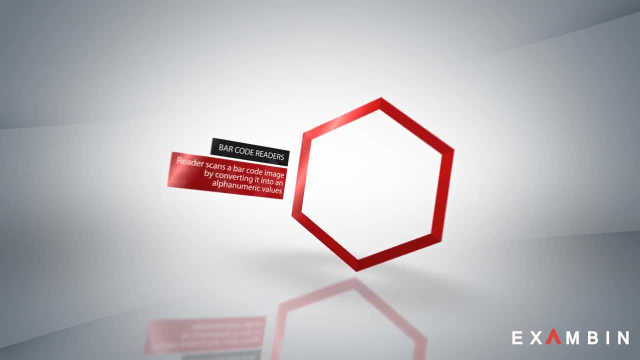 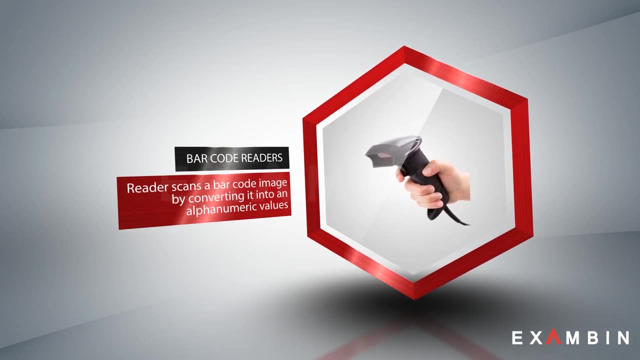 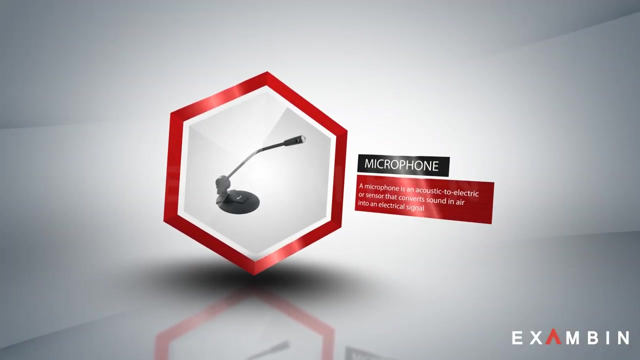 called integrated circuit cards. Barcode readers are used for reading barcoded data. Barcode reader scans a barcode image by converting into an alpha numeric values. Microphone: A microphone is an acoustic to electric transducer or sensor that converts sound in air into an electrical signal. 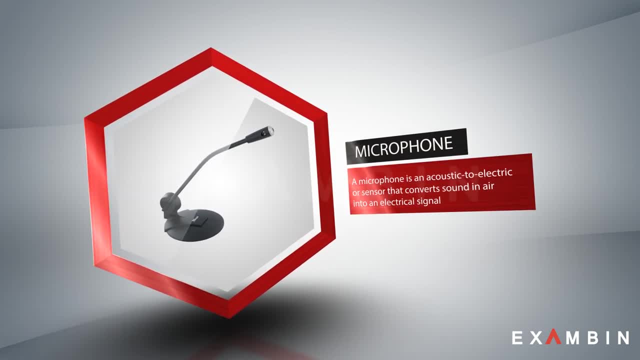 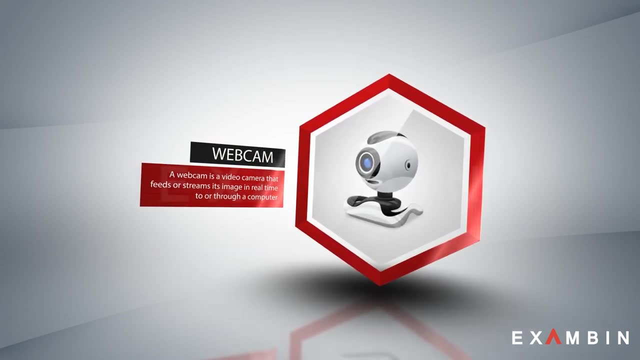 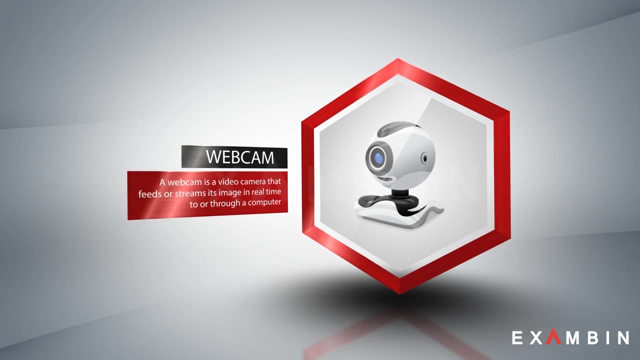 Microphones are used in many applications, such as telephones, hearing aids, mobile phones, etc. Webcam. A webcam is a video camera that feeds or streams its image in real time to or through a computer network. When captured by the computer, the video stream may be saved, viewed or sent on to other networks. 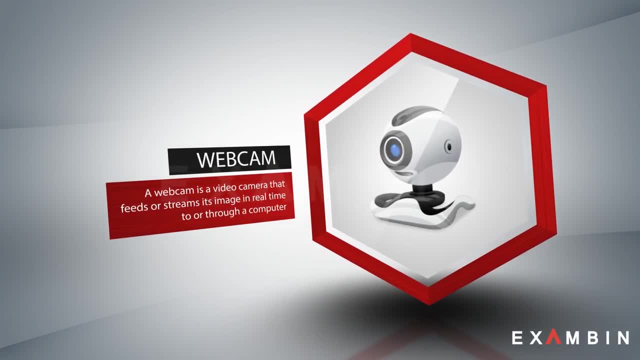 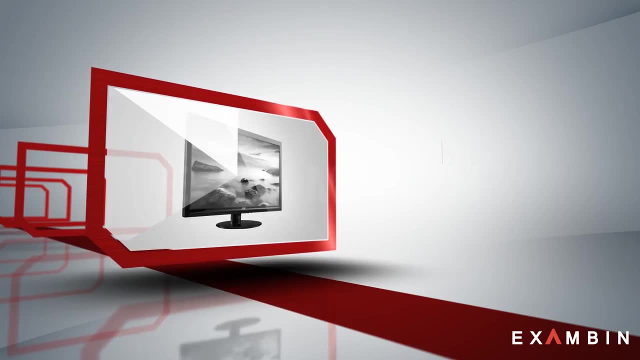 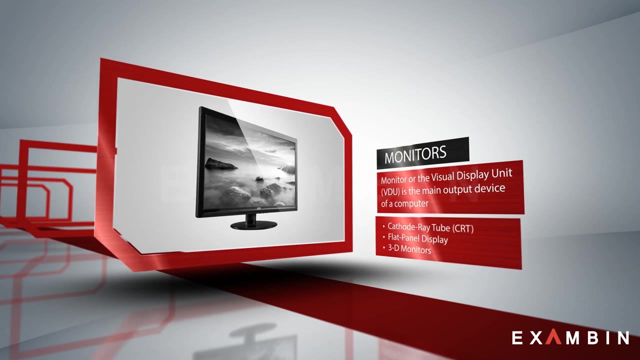 via systems such as the internet, An email as an attachment. We will now see some major output devices: Monitors. Monitors, or the visual display unit, is the main output device of a computer. It forms images in the form of tiny dots known as pixels.